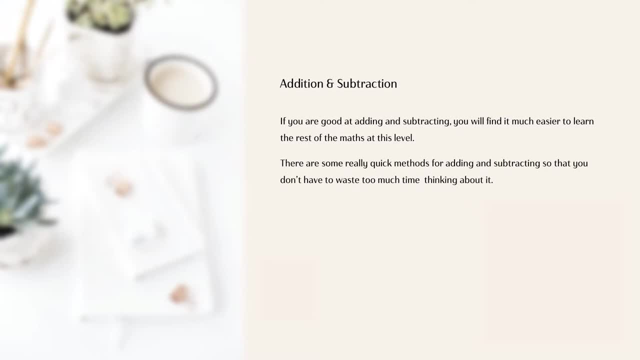 to learn the rest of the maths at this level. There are some really quick methods for adding and subtracting so that you don't have to waste too much time thinking about it. 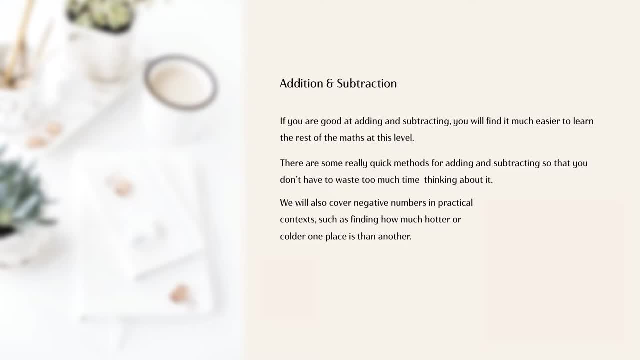 We will also cover negative numbers in practical contexts such as finding out how much hotter or colder one place is than another. For some questions you will not be able to use a calculator 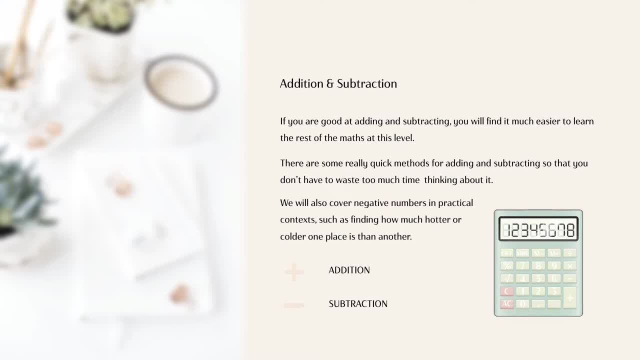 but for others you will. When using a calculator, it helps to estimate your answer first. This way if you press an incorrect button and the answer is way off, you should realise and carry out your calculation again. 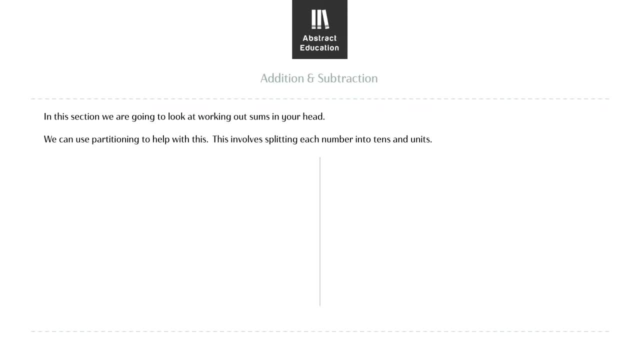 In this section, we are going to look at working out sums in your head. We can use partitioning to help with this. This involves splitting each number into tens and units. Here is an example of addition. 32 plus 46. 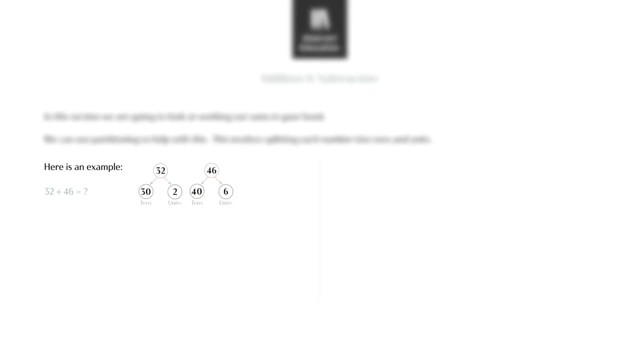 If we first split each number into tens and units, it should look something like this. We can add the tens first. 30 plus 40 equals 70. Then add the units. 2 plus 6 equals 8. 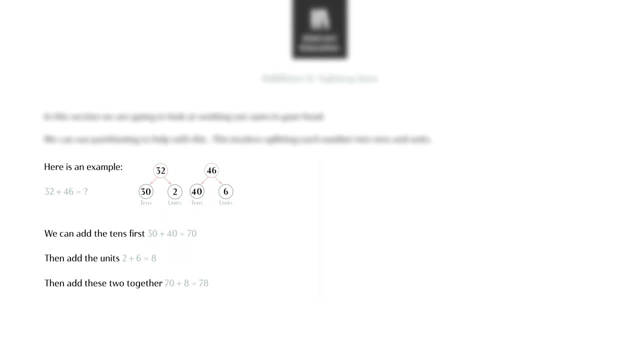 Then add these two together. 70 plus 8 equals 78. Here is an example of subtraction. 56 minus 34. 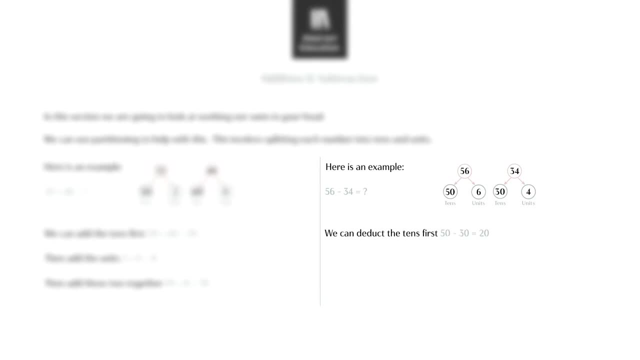 We can deduct the tens first. 50 minus 30 equals 20. Then deduct the units. 6 minus 4 equals 2. Then add these two together. 20 plus 2 equals 22. 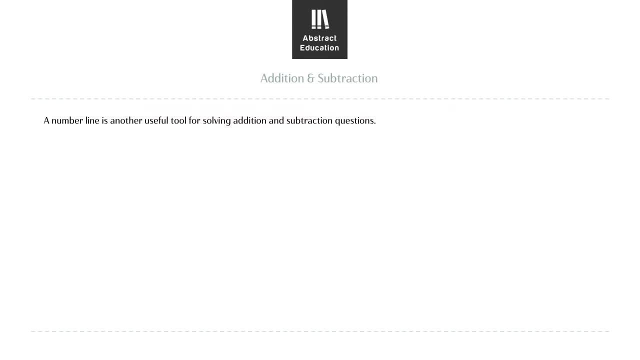 A number line is another useful tool for solving addition and subtraction questions. Work out 145 minus 68. 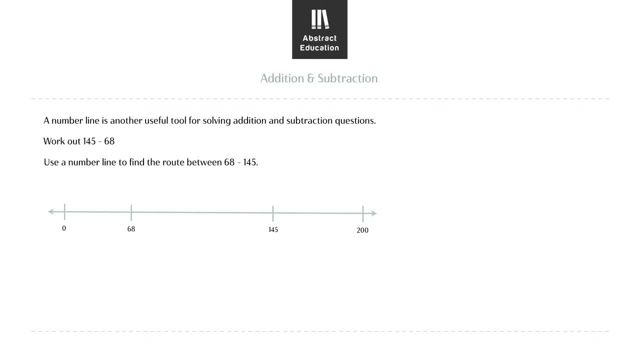 145 minus 68. But we can use a number line to find the route between 68 and 145. If we count from 68 to 70, this leaves the number 2. We then count from 70 to 100, which leaves 30. From 100 to 145, this leaves 45, and therefore we need to add 2 plus 30 plus 45. This equals 77. 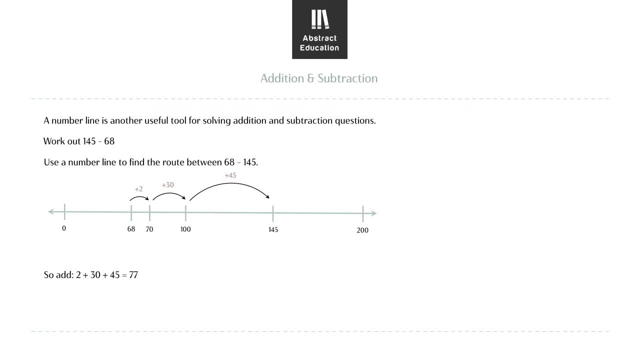 A number line can be extended infinitely in any direction and is usually represented horizontally. 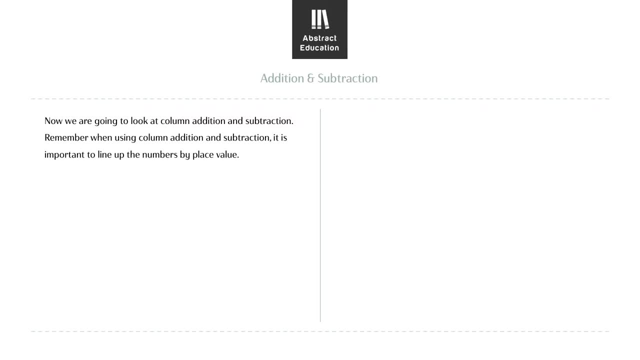 Now we are going to look at column addition and subtraction for those larger numbers. If the numbers are too high or too difficult to add or subtract in your head, we can write them down in columns. 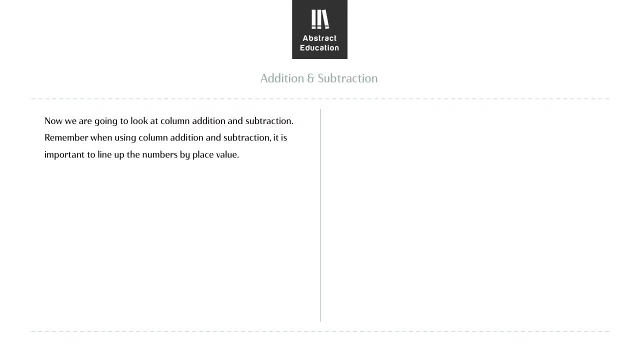 It is important to first separate the numbers into ones, tens, hundreds and thousands, etc. Let's look at the example 2367 plus 452 plus 85. 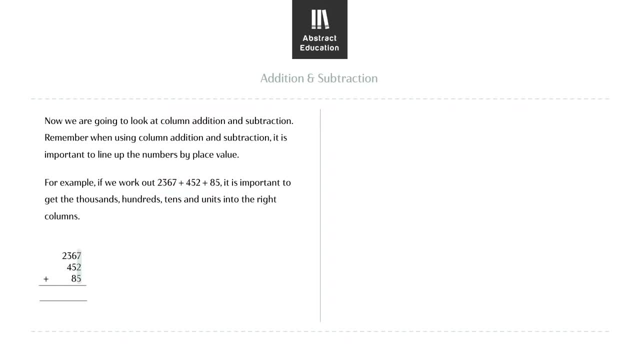 We must always add up the units column first. So 7 plus 2 plus 5 equals 14. Because our answer has gone from one digit to two, we take the unit which is four and write this in the answer underneath the column of units. We can then carry one over to the tens. Now add up the tens column. So 6 plus 5 plus 8 which equals 19. Before we put the answer in, we must add the leftover unit of 1 to the total. So this makes 20. 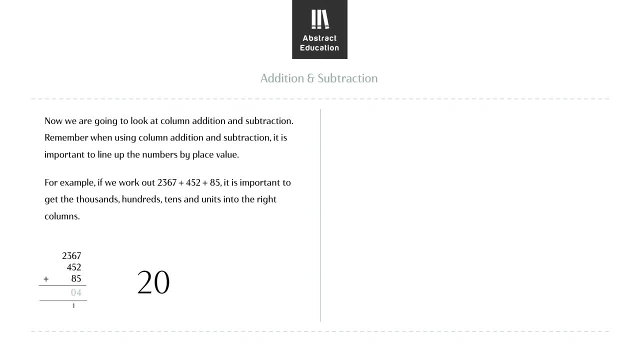 So we now put the 0 in the answer under the tens column and carry the 2 over to the hundreds. Next we add up the hundreds column. 3 plus 4 equals 7. 7 added to the tens column. 7 added to our leftover 2 equals 9 and therefore, we put this answer in. The next column has one number which is 2 and there is nothing else carried forward. Therefore, we place 2 in the answer. The total answer is now 2,904. 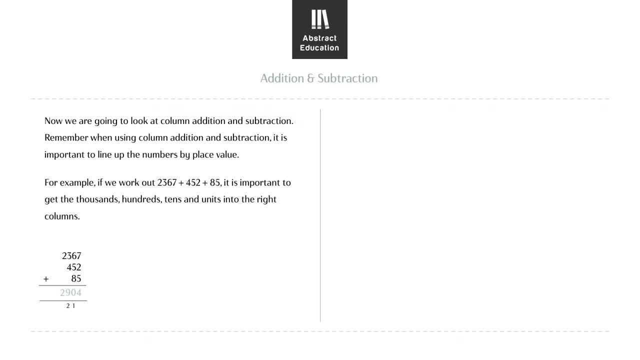 Now that we have tried column addition, we will now look at column subtraction. 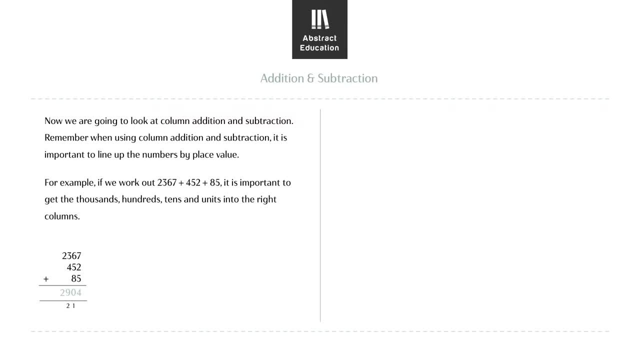 This is an efficient method, but you must have an awareness of place value. Let's work on column subtraction. 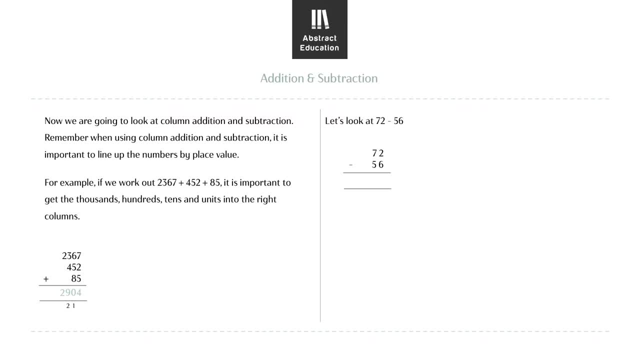 We will work out 72 minus 56. First we line up our units and tens columns, then we subtract the units column. 6 is greater than 2 and in order to deduct 6 from 2, we must borrow 1 from the tens. We therefore cross out 7 and change it to 6 and transfer the 1 over. Now we deduct 6 from 12 which equals 6. This is written into the answer column. Next we deduct 5 from 6 which equals 1. 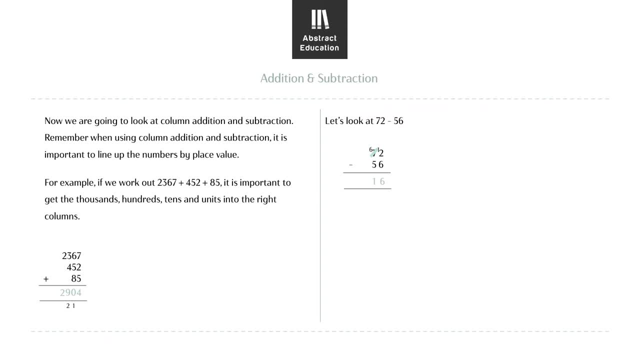 Now that we have covered adding and subtracting whole numbers, we will move on to decimals. 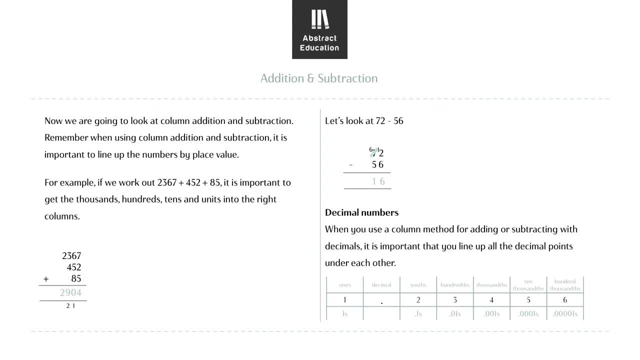 When you use a column method for adding or subtracting with decimals, it is important that you line up all the decimal points under each other. 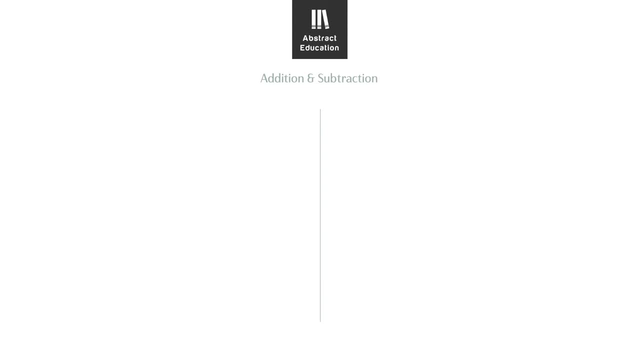 We are going to have a look at an example on the next page. Here is an example. 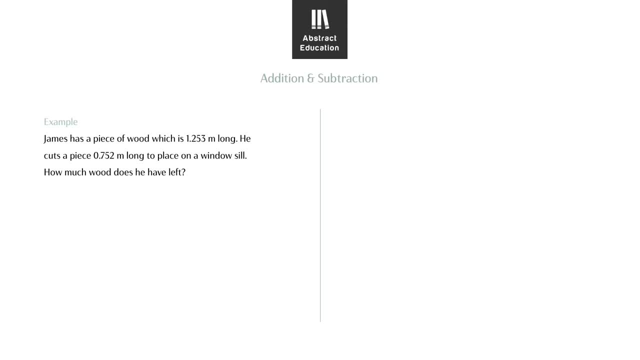 James has a piece of wood which is 1.253 metres long. He cuts a piece which is 0.752 metres long and it is to place on a windowsill. How much wood does he have left? 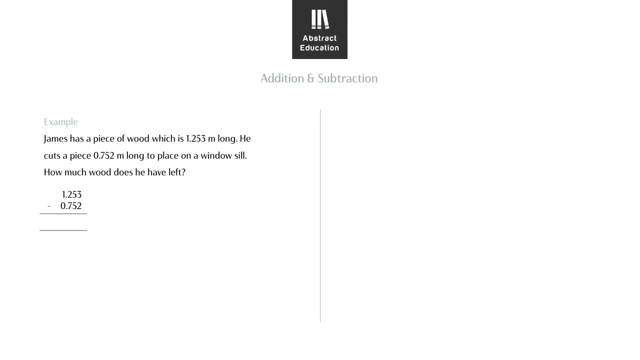 First find the sum you need to answer. So that's 1.253 metres minus 0.752. 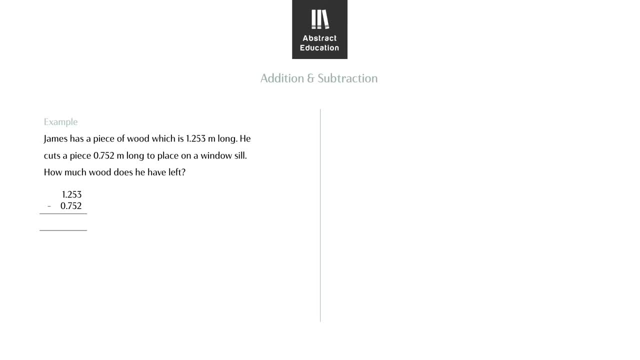 Now write it in column format. Now we are going to carry out the calculation which is very similar to the one previously. Beginning with the thousands column, 3 minus 2 equals 1. 5 minus 5 equals 0. For 2 minus 7, we must take 1 from the units column making our calculation 12 minus 7. This equals 5. Then 0 minus 0 equals 0. So our answer is 0.501. 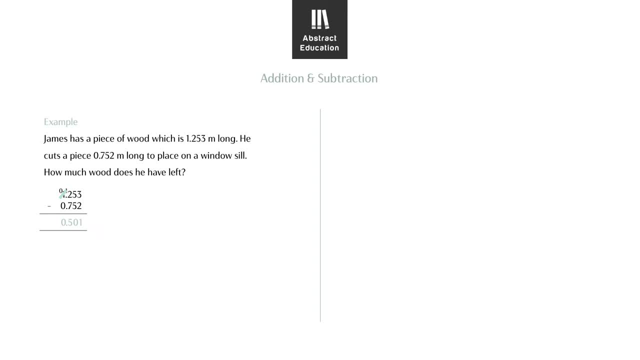 When you add or subtract decimals, make sure you line up the columns correctly. The decimal points in the numbers you are working with and the answer should be underneath each other with the numbers matching each place value. This includes zeros. 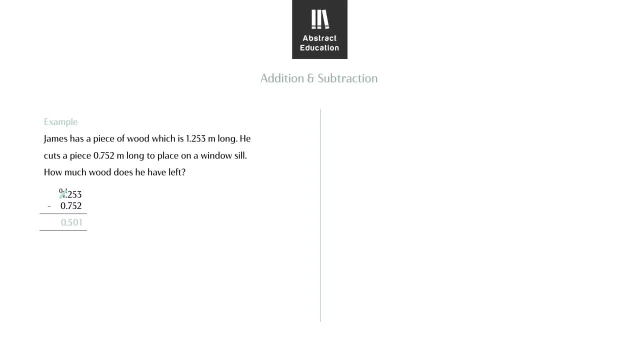 With problems, you will need to decide whether the amounts involved should be added or subtracted. Here are some examples of the words you should look for. 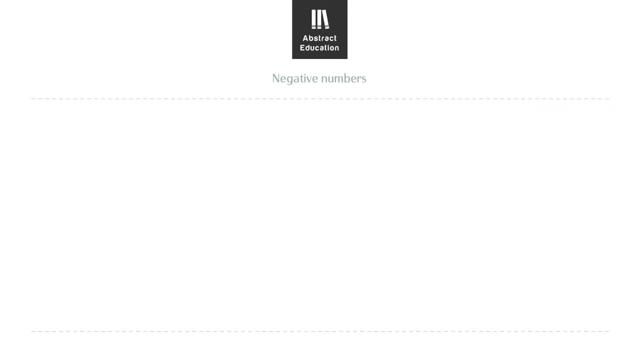 Ok, so we do cover negative numbers in a previous video, but we are going to just briefly cover it also in this one. We want you to be able to use negative numbers in practical circumstances. You will need to add to them or subtract from them. Negative numbers are numbers less than zero. 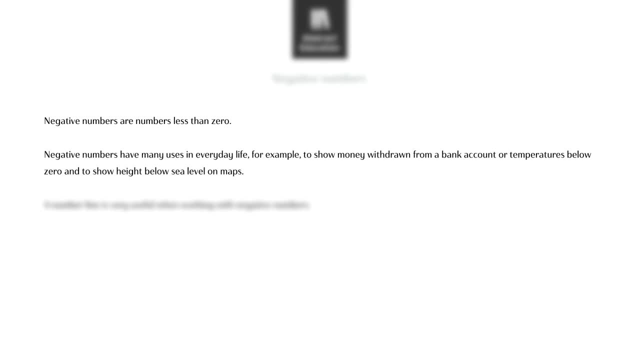 Negative numbers have many uses in everyday life. For example, to show money withdrawn from a bank account or temperatures below zero and to show height above sea level on maps. 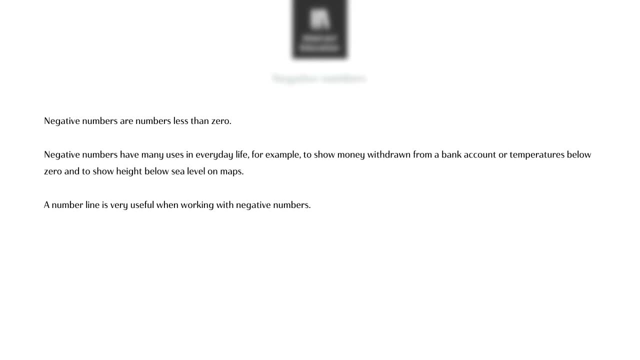 A number line is a very useful tool when working with negative numbers. If you look at the number line, you will notice that the further to the left a number is, the smaller it is. 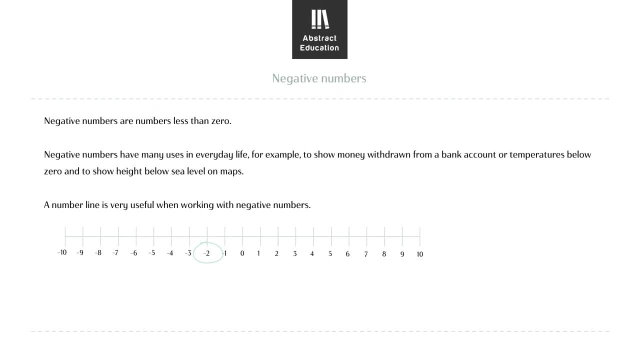 For example, minus 2, we say negative 2 or minus 2 and this is smaller than 1. Negative numbers are often used when talking about temperature. 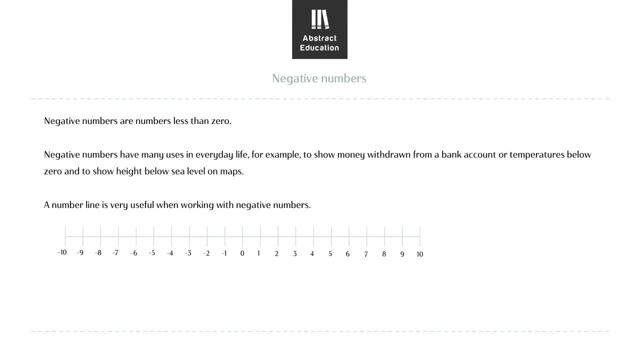 For example, on a cold winter's day, the weather forecast might give the temperature as below freezing or minus 2. 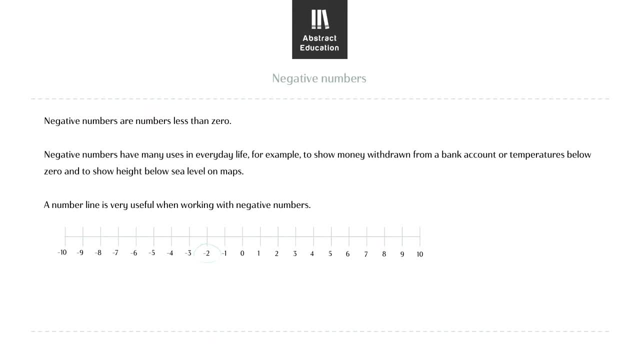 The temperature of a freezer would also be a negative number. Negative numbers can also be used to talk about money. 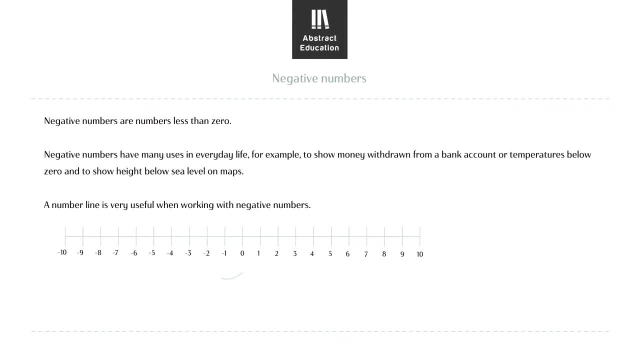 Think of the amount of money you have in your bank account. If you go into minus numbers, this means you owe money. So, minus 2 means you owe £2. 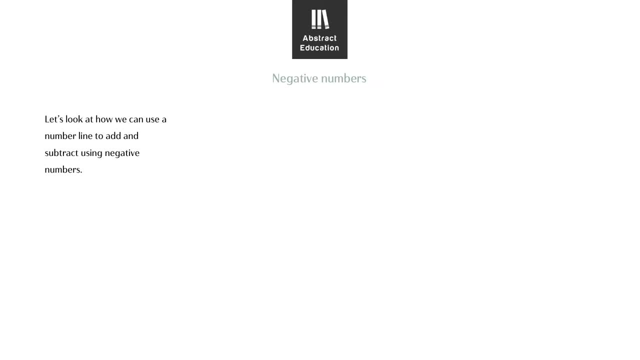 Let's look at how we can use a number line to add and subtract using negative numbers. First, draw a number line and find your starting point which is zero. Next, you need to count 6 to the right. Here is how you would add 3 and finally here is how you would subtract 6. 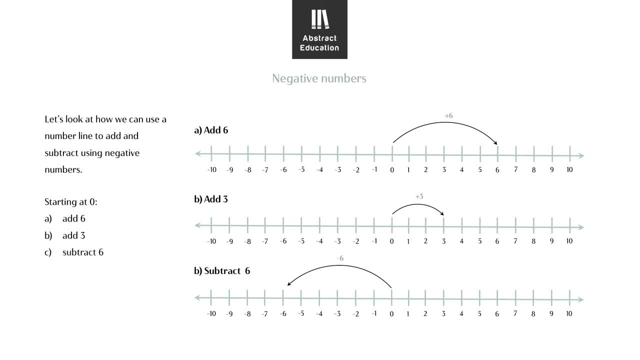 Having a picture in your head of a number line above and below 6 and below 0 is really useful for this type of question. You can imagine bouncing along it as you add or subtract. 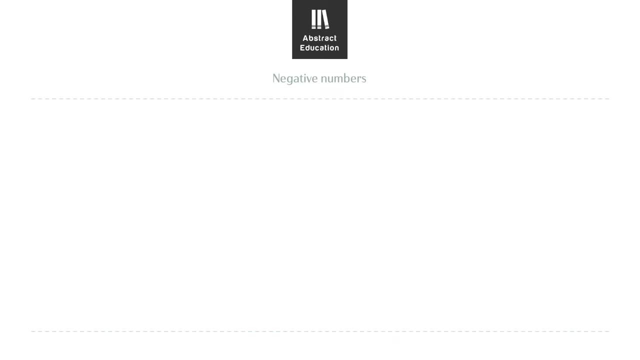 Here is a practical scenario which uses negative numbers. The temperature at 6pm is 1 degrees. By 4am the next day, it has fallen 4 degrees. What is the temperature? We must begin by drawing our number line and counting down from 1 degrees. Our answer is minus 3 degrees. 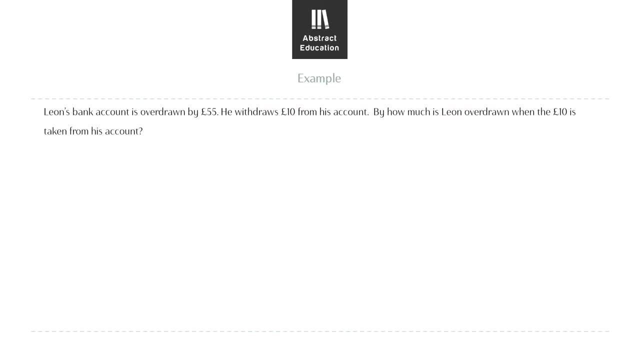 Here is another example. Leon's bank account is overdrawn by £55. He withdraws £10 from his account. By how much is Leon overdrawn when the £10 is taken from his account? The bank account is already £55 overdrawn which means there is minus £55 in Leon's bank account. If he withdraws another £10, then the account will be overdrawn by £55 plus £10. This equals minus £65. Leon is overdrawn by £65. We are now moving on to multiplication and division. 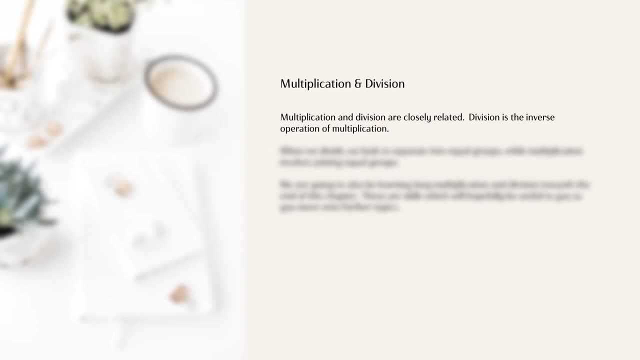 Multiplication and division are closely related. Division is the inverse operation of multiplication. When we divide, we look to separate into equal groups, while multiplication involves joining equal groups. 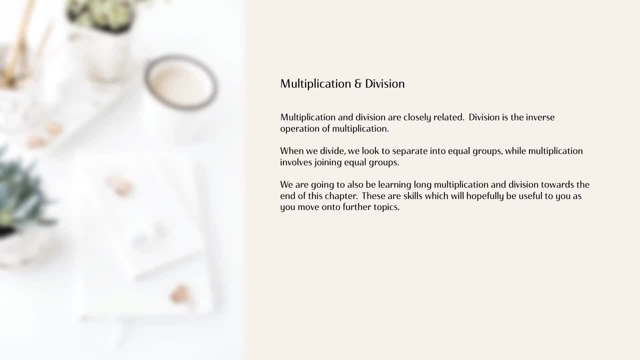 We are going to also be learning long multiplication and division towards the end of the chapter. These are skills which you will hopefully find useful as you move on to further topics. Here we are going to look at some basic calculations. 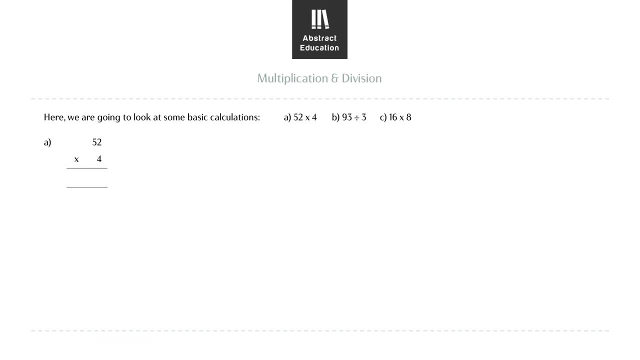 For question A, we have 52 multiplied by 4. To begin, we must first multiply the units by 4 and then the tens by 4. 2 times 4 equals 8 and 5 times 4 equals 20. 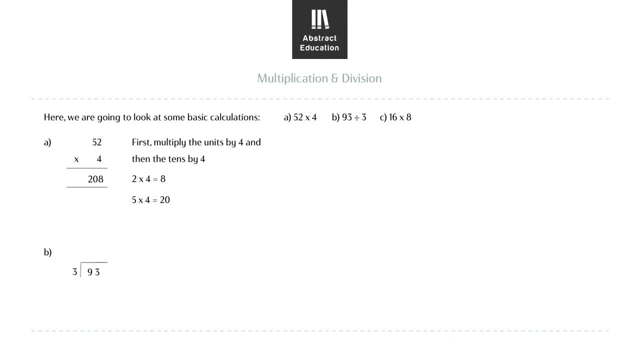 93 divided by 3. First divide the tens and then the units by 3. 9 divided by 3 equals 3. 3 divided by 3 equals 1. 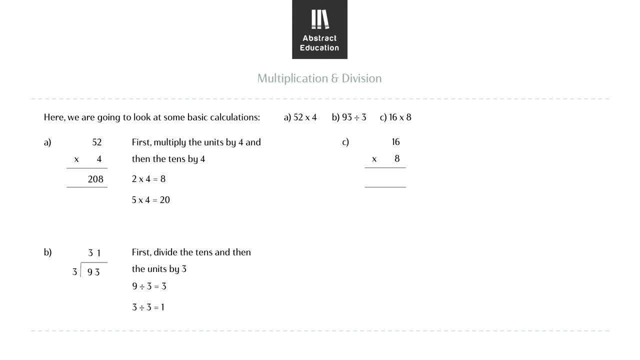 16 multiplied by 8. 6 times 8 equals 48. You write the 8 in the units column and carry 4 tens over. 1 times 8 equals 8. Add 8 to the remainder of 4, which is 12. 100 is carried over. 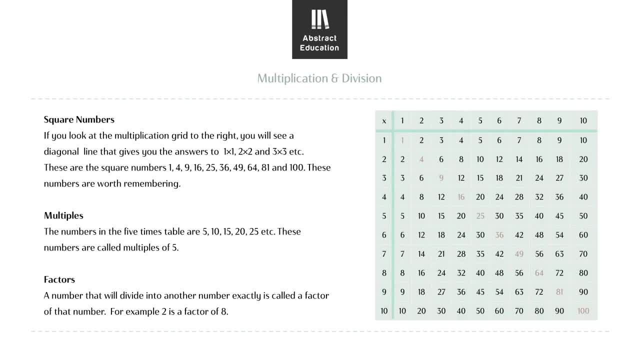 If you look at the multiplication grid, you will see a diagonal line that gives you the answers to 1 times 1, 2 times 2 and 3 times 3, etc. These are the square numbers, so 1, 4, 9, 16, 25, 36, 49, 64, 81 and 100. These numbers are worth remembering. There are also numbers which are classed as multiples. An example would be the numbers in the 5 times table. They are 5, 10, 15, 20, etc. These numbers are called multiples of 5. Lastly, there are factors. 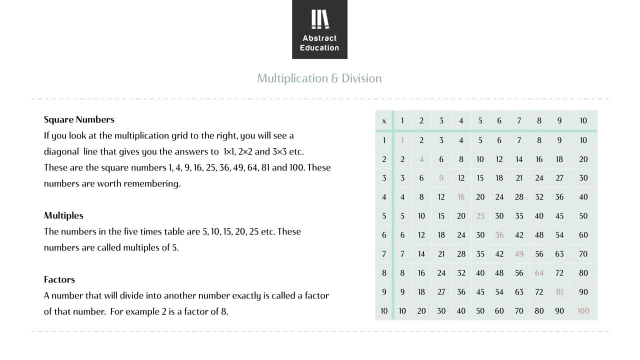 A number that will divide into another number exactly is called a factor of the number. So, for example, 2 is a factor of 8. 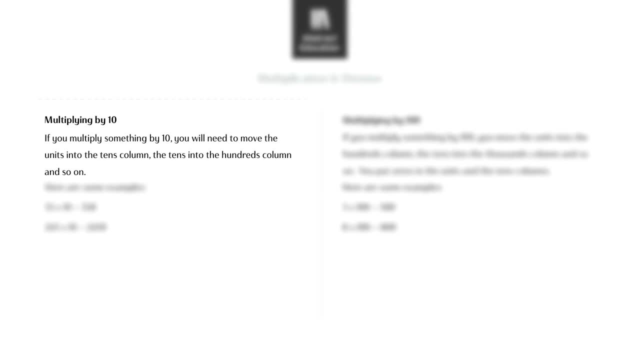 If you multiply something by 10, you will need to move the units into the tens column, the tens into the hundreds column and so on. Here are some examples. 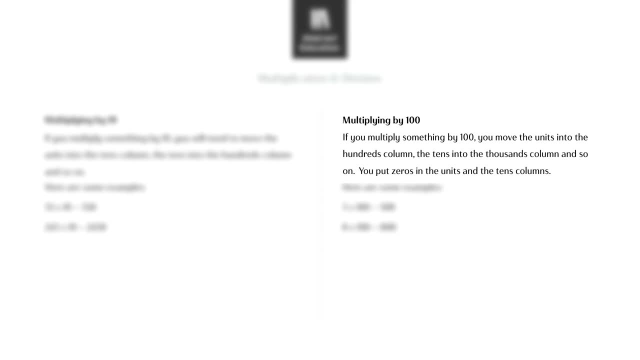 If you multiply something by 100, you move the units into the hundreds column, the tens into the thousands column and so on. Here are some examples. 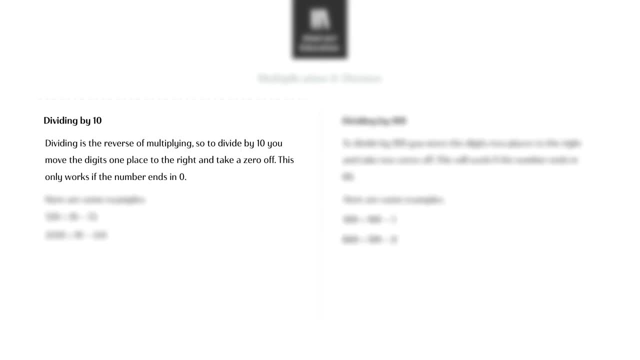 Dividing is the reverse of multiplying. So, to divide by 10, you move the digits one place to the right and take a zero off. This only works if the number ends in zero, though. Here are some examples. 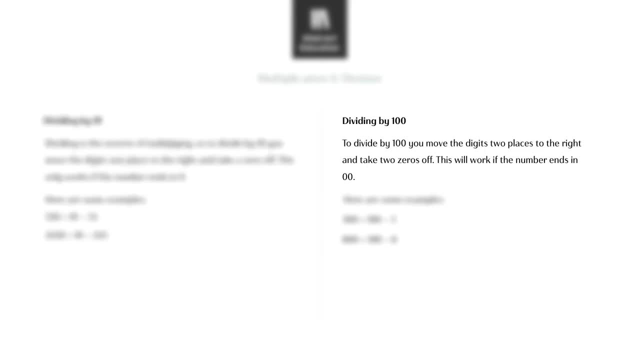 To divide by 100, you move the digits two places to the right and take the two zeros off. This will work if the number ends in 00. Here are some examples. 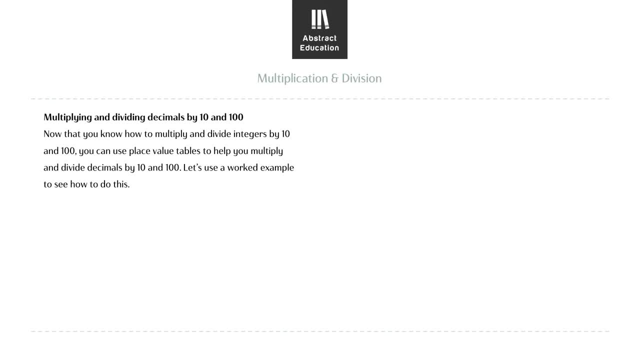 You can use place value tables to help you multiply and divide decimals by 10 and 100. Let's use a worked example to see how to do this. So, 25.7 multiplied by 10. To multiply by 10, you move each digit one place to the left. So, 25.7 multiplied by 10 equals 257. 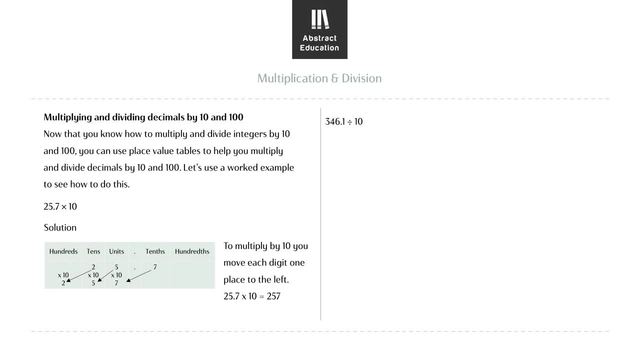 Let's look at 346.1 divided by 10. To divide by 10, you move each digit one place to the right. 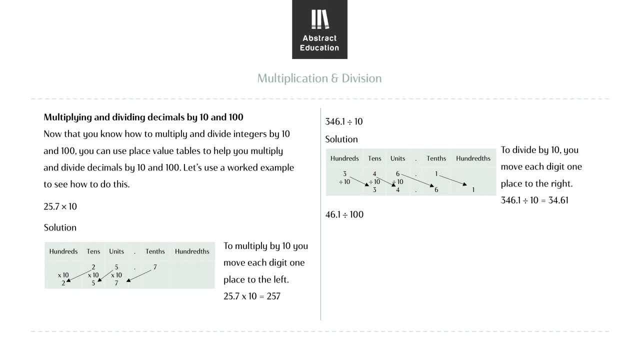 So, to divide by 100, you move each digit two places to the right. 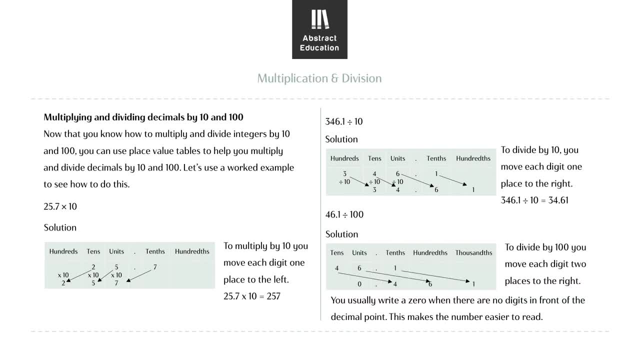 You usually write a zero when there are no digits in front of the decimal point. This makes the number easier to read. 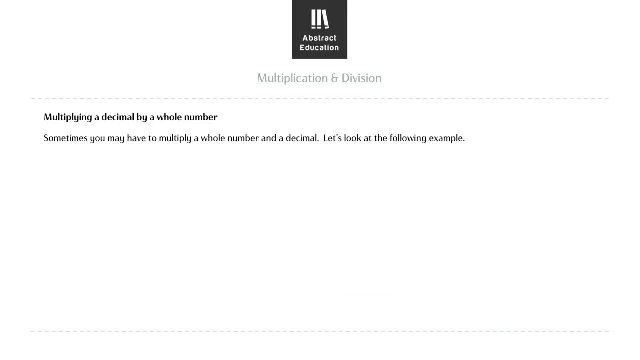 Sometimes you may have to multiply a whole number and a decimal. Let's look at the following example. 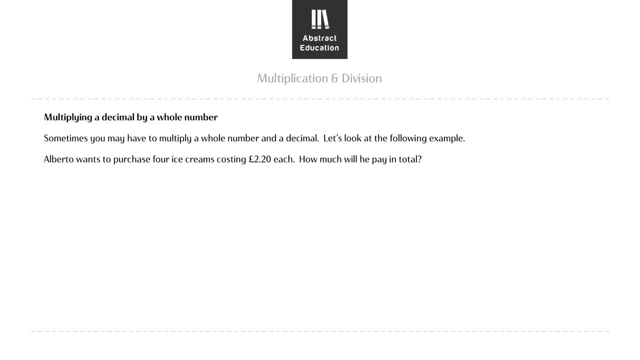 Alberto wants to purchase four ice creams costing £2.20 each. How much will he pay in total? 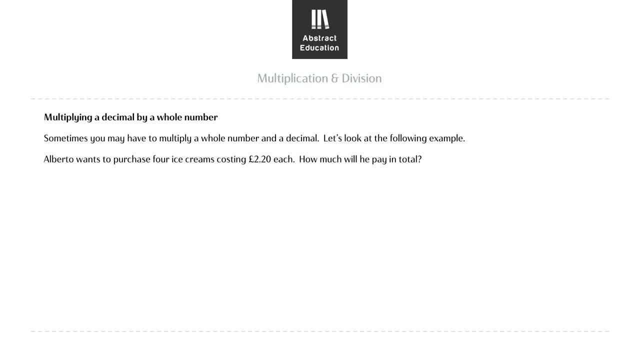 There are two ways of doing this. We can either work in pence or pounds. I will show you both methods. So, working in pence. Your calculation should look like this. First, you multiply the units. Zero times three equals zero. Then the tens. Two times three equals six. Then the hundreds. Two times three equals six. 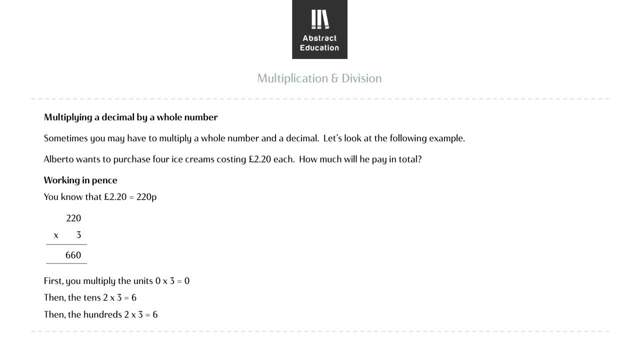 Your answer is 660, which can then be converted into £6.60. 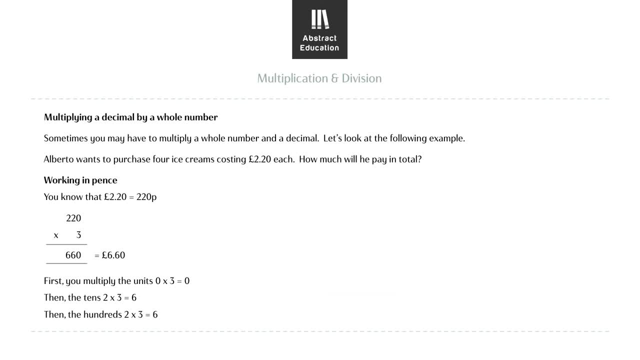 Now we will work in pounds. The answer is £6.60. 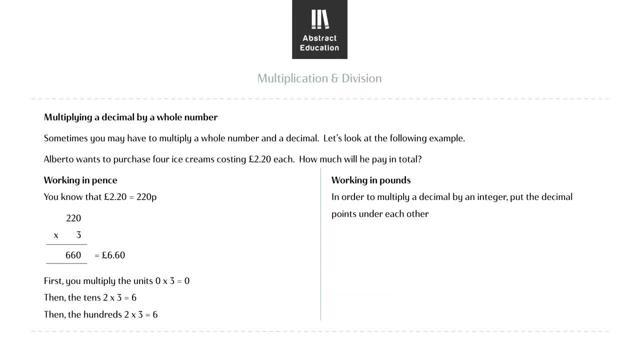 Make sure you line your work up carefully by placing the decimal points in line underneath one another. So, zero multiplied by three equals zero. 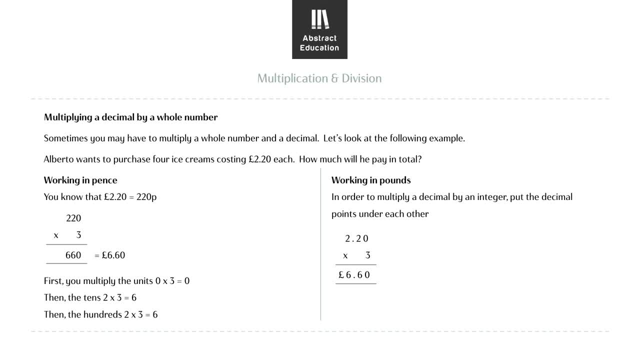 And two multiplied by three equals six. And finally, two multiplied by three equals six. 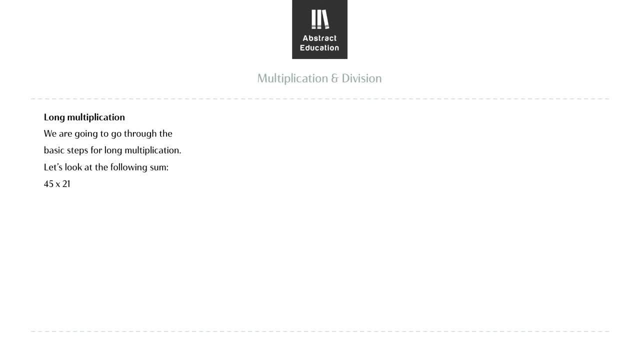 Here we explain the basic steps for long multiplication. Let's look at the following sum. First we need to put the digits into columns and line them up. The five and one are aligned in the units column. And the four and two are aligned in the tenths column. We will start by multiplying the number at the bottom with the one at the top. We always begin by multiplying the units. So, one multiplied by five equals five. 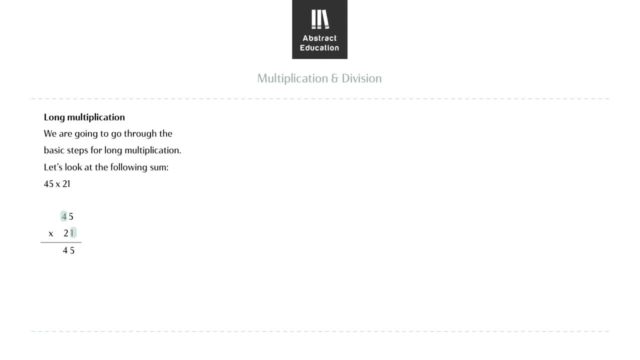 We will then multiply one by the digit in the tens column. So, one multiplied by four equals four. 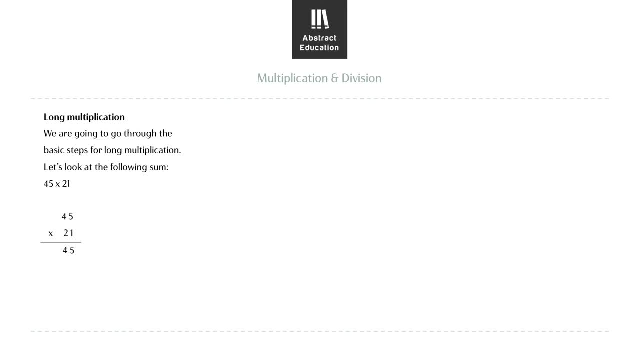 We have now multiplied the units digit of the bottom number with each of the digits of the top number. 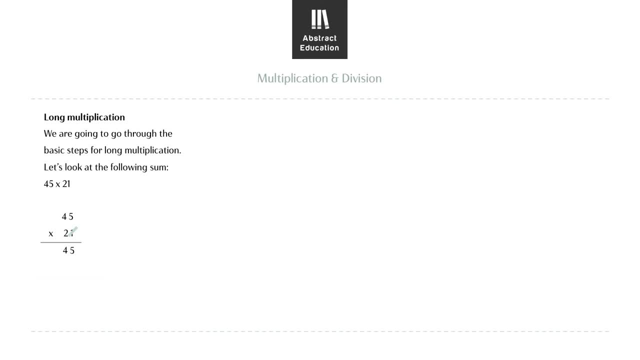 We can strike out this digit. We will now move on to the next digit for the bottom number, which is in the tens column. 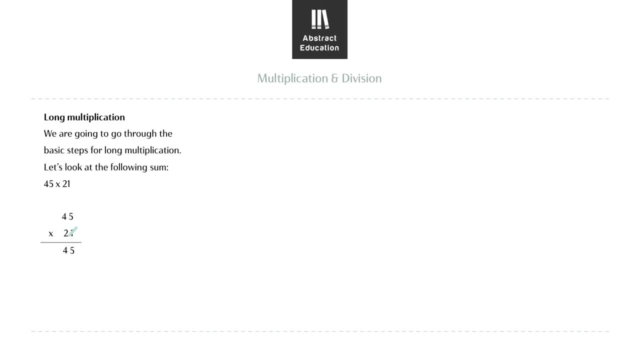 Because the tens digit always has a units digit next to it, we will need to add a zero to the units column. 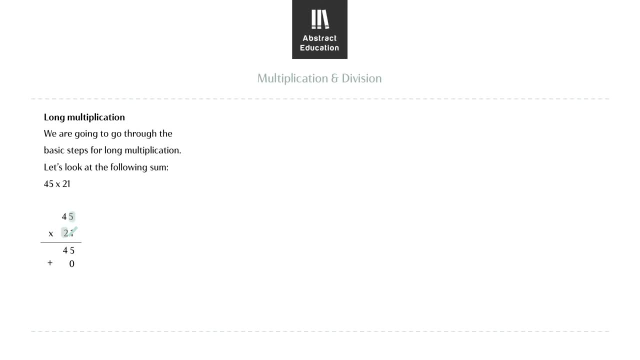 So, two multiplied by five equals ten. So, zero is written in the tens column. 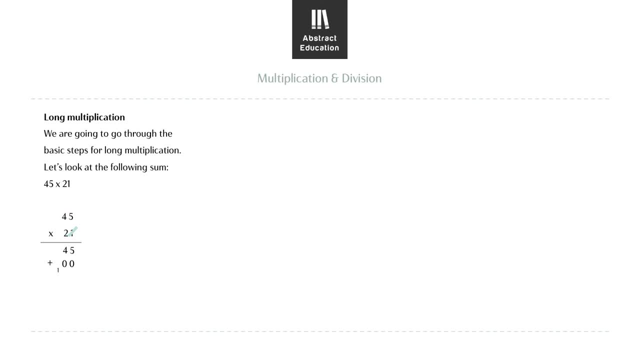 And one is carried over to the hundreds column. Our next calculation is two multiplied by four, which equals eight. We then add eight to our remaining one, which is carried over. This equals nine, which is placed in the hundreds column. The final step is to add both answer columns together, which gives us our answer. Nine hundred and forty-five. 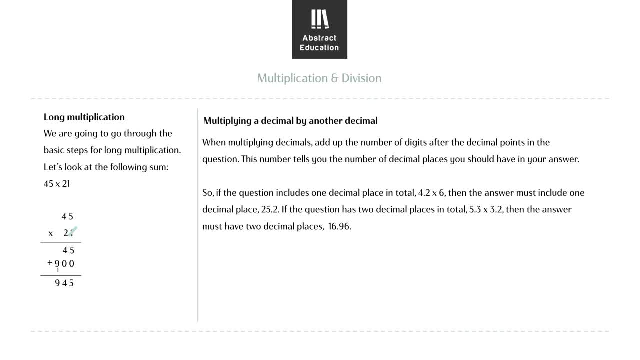 When multiplying decimals, add up the number of digits after the decimal points in the question. This number tells you the number of decimal places you should have in your answer. 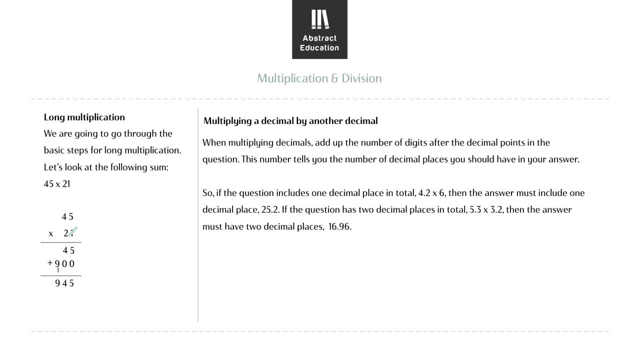 So, if the question includes one decimal place in total, four point two multiplied by six, then the answer must include one decimal place, twenty-five point two. 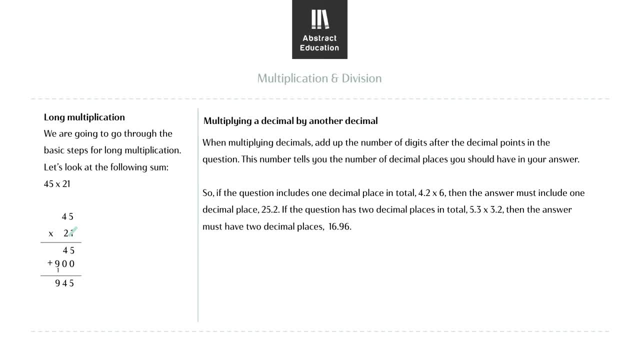 If the question has two decimal places in total, five point three multiplied by three point two, then the answer must have two decimal places, sixteen point nine six. 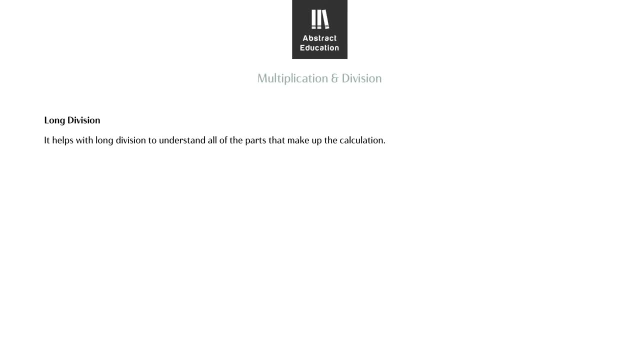 It helps with long division to understand all of the parts that make up the calculation. 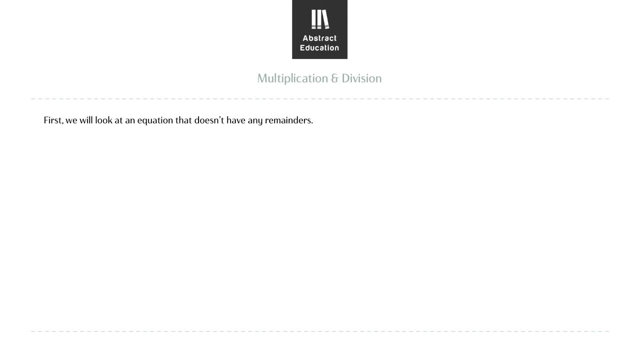 First, we will look at an equation that doesn't have any remainders. 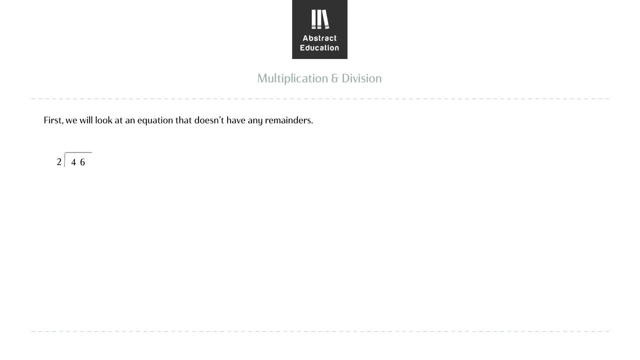 Forty-six divided by two. How many times does two go into four? The answer is two, and this is written above the four. 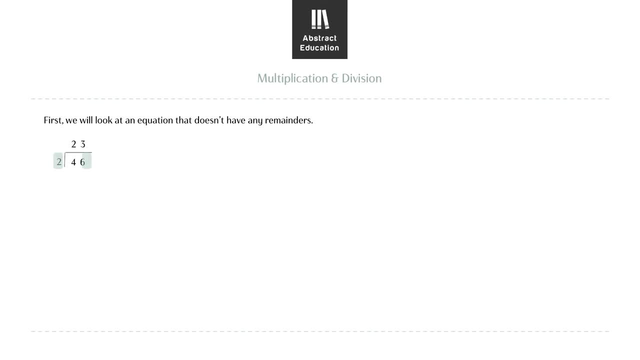 Next, we work out how many times two goes into six. The answer is three, and this is written above. Our answer, therefore, is twenty-three. 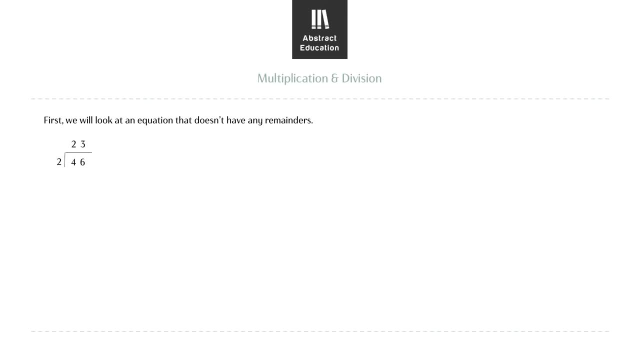 Once you are confident dividing in the basic format, we can then move on to division with remainders. 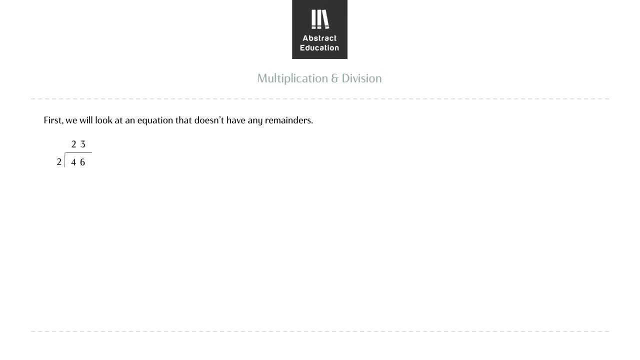 In mathematics, the remainder is the amount left over when the first number does not divide exactly by the other. 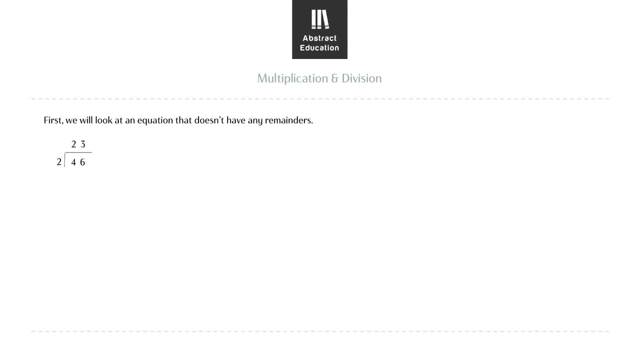 For example, say you have a two hundred centimetre length of wood. 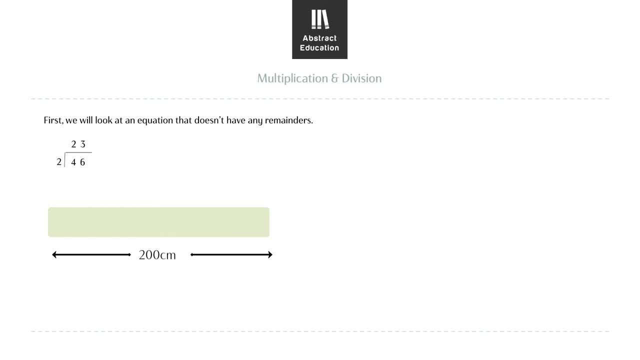 How many lengths of sixty centimetres can be cut off from this length? When you do two hundred divided by sixty, you get three whole sixty centimetre lengths, which measures a hundred and eighty centimetres in total, and so you have a remainder of twenty centimetres left. Let's look at the following example. 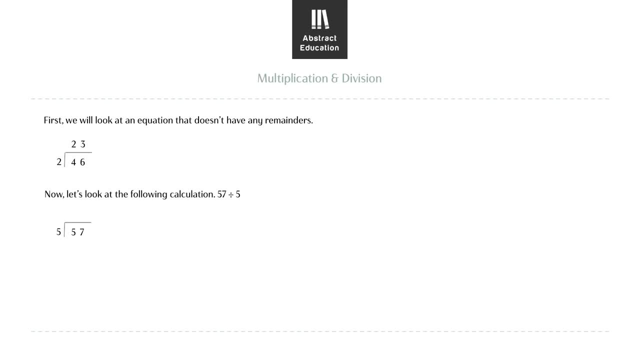 Fifty-seven divided by five. We begin with the tens column, and five goes into five once. Therefore, we write one in the answer above. Next, we need to work with the units column, which is seven. If we try to work out how many times five goes into seven, we know that it will go once, but there will be a remainder. 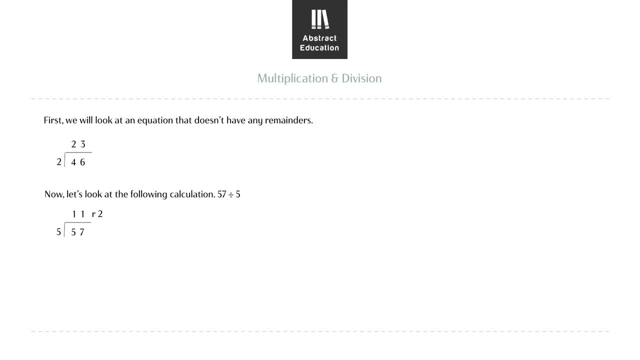 The remainder is two, and therefore your answer will look like this. Eleven remainder two. 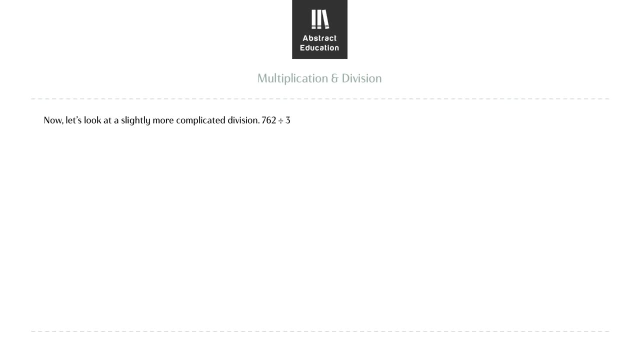 Now let's look at a slightly more complicated calculation, which we will carry out long division for. Seven hundred and sixty-two divided by three. The steps you must remember when carrying out long division are... 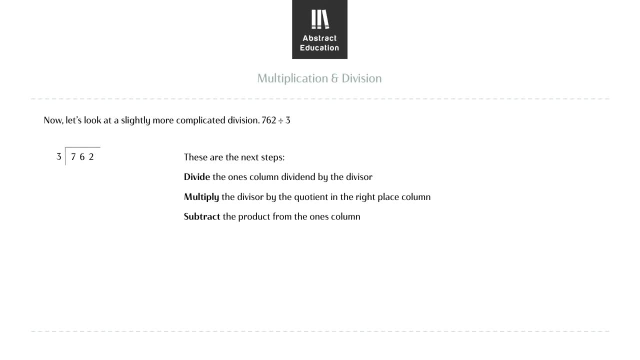 The first step is to see how many times three will go into seven. So seven divided by three equals two remainder one. 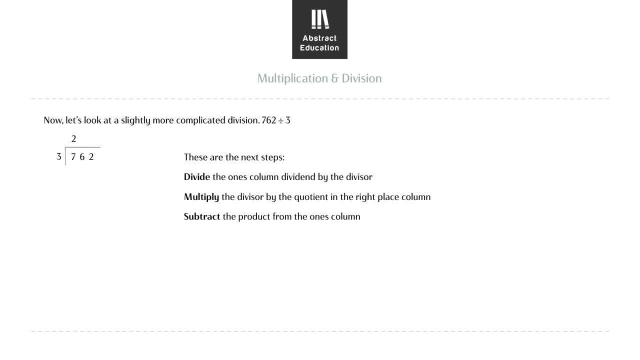 We write the two above the seven, and we will see the remainder one later on. 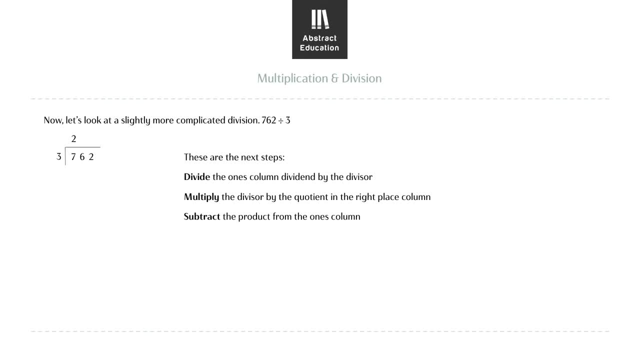 Next, we multiply two by three. So two times three equals six. The answer six is placed below the seven. Now we subtract the six from the seven. So seven minus six equals one. One is our remainder. As you can see above, 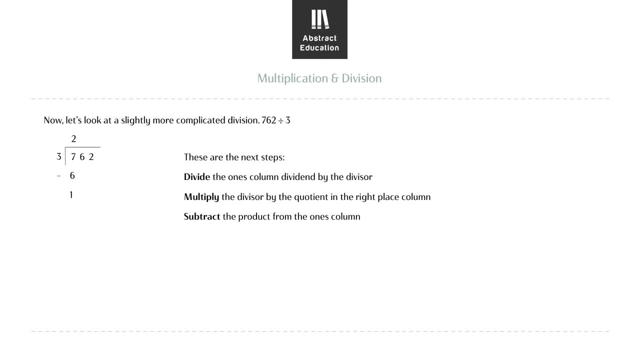 we have gone through the process of dividing, multiplying and subtracting the three. 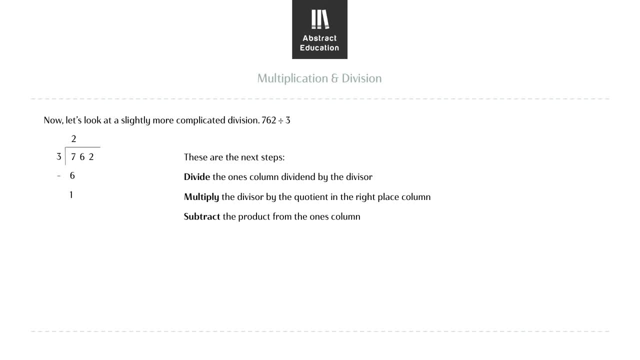 And subtracting the first digit of our dividend. We now go through that process with the next digit of six. But first we must bring the six down, so that it is in line with our first answer of one. This now makes the digit sixteen. Sixteen divided by three equals five remainder one. Ignore the remainder for now, and answer with five. Five multiplied by three equals fifteen. 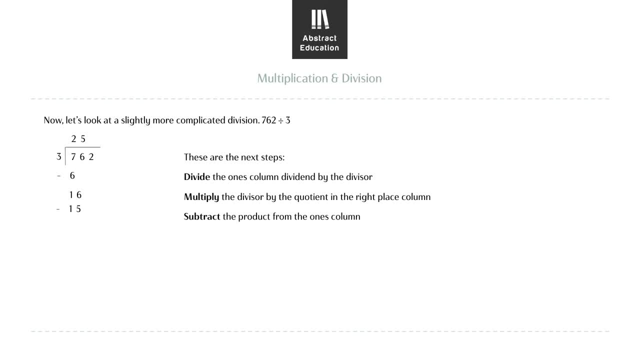 Write fifteen directly beneath the sixteen. 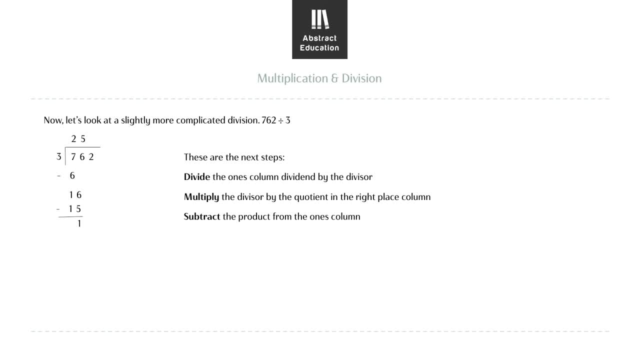 Sixteen minus fifteen equals one. Now you subtract and the answer is one. 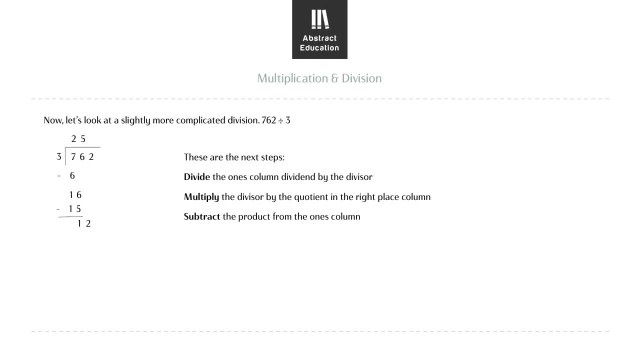 Next bring down the two, making your latest answer twelve. 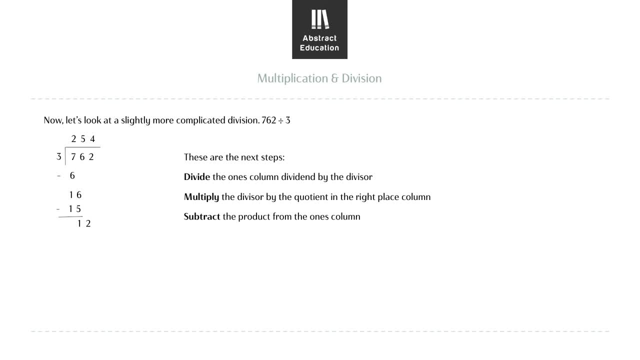 And twelve divided by three equals four. Write your answer at the top. Four multiplied by three equals twelve. So write twelve beneath your answer. 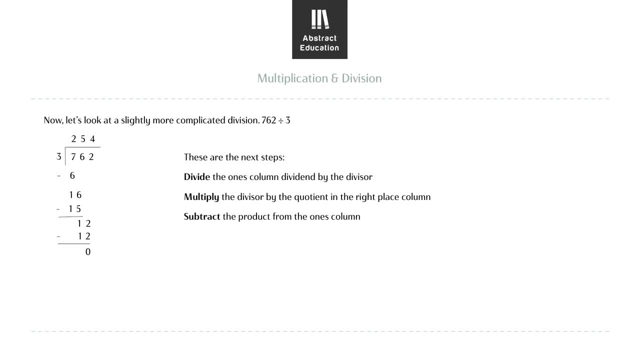 Twelve minus twelve equals zero. So you are left with no remainders. Your answer is two hundred and fifty-four. 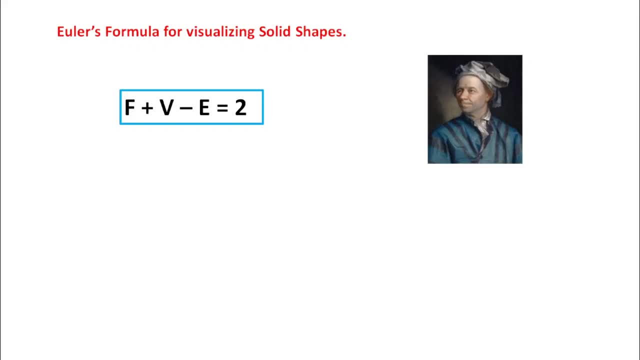 Hello everyone, welcome to Definite Mind. In this video session, we are going to know about a formula which was given by Leonard Euler- and he was a great mathematician- and he gave this formula to visualize solid shapes such as pentahedron, cube, cuboid and prism pyramid. also, 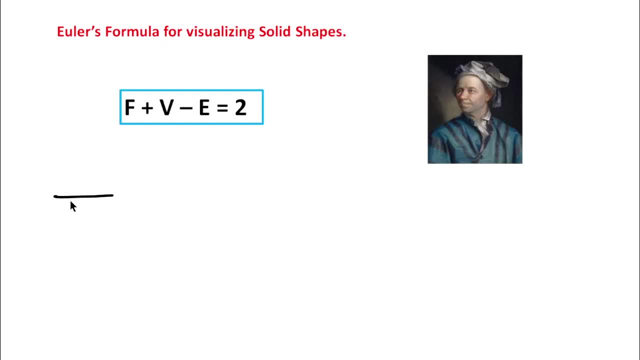 Let's suppose this is a cuboid. In this cuboid, how many faces are there: Top, bottom, left, right and this side? and this side? Ok, Means there are total 6 faces, f equal to 6, and how many vertices? 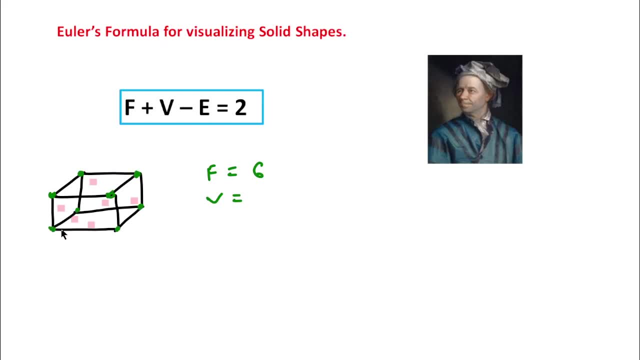 4 in top and 4 in bottom. This means total 8 vertices and how many edges? 1,, 2,, 3, 4.. 4 in top and 4 in bottom. 4 plus 4 is 8, and 8 to 10 and 10 to 12..